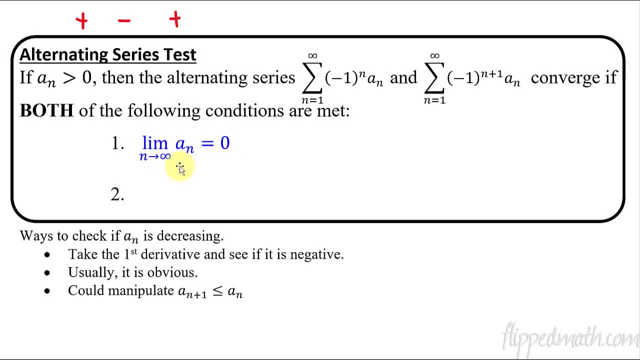 then here's the two conditions. The first one is that the limit as n approaches infinity, of this a of n, here this function is going to equal zero. That's the first condition. If the limit doesn't equal zero, then it's not going to well, we can't say that it converges. Now the 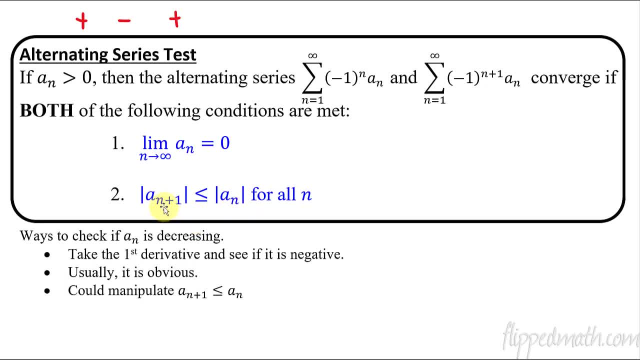 second condition here is this, and that is that the succeeding term is smaller than the previous term. So, in other words, if you have the first term, the second term will be smaller, For if you have the third term, the fourth term is going to be smaller. So if you have the third term, the fourth term is going to be smaller. 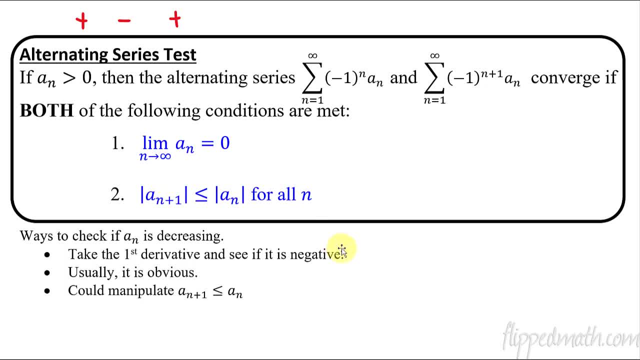 The one that comes next, Or in other words, this is just a fancy way of saying that it is decreasing, that these things are decreasing. Now why the absolute value? I put the absolute value there just to make sure that you understand like it's. we're not confusing it. 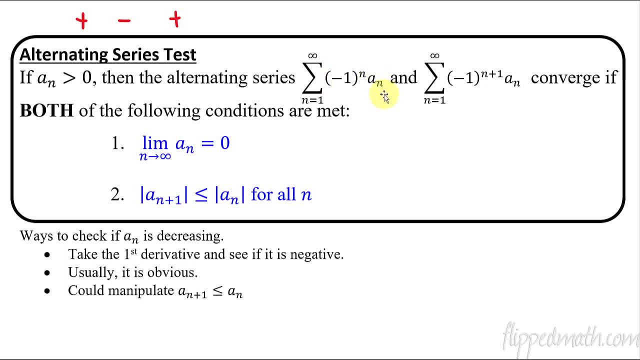 with the negative, Like if you, sometimes students will apply the negative one. Technically I don't need to put those absolute values there, because I've already said here that it's got to be positive, but I'm putting them there. A lot of times you'll see textbooks do that, uh, just to reference that. 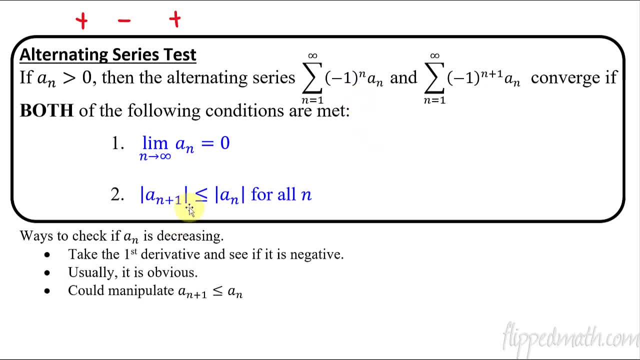 it's the entire thing. So we don't care that it's positive or negative. You just take the absolute value and the next term is going to be smaller than the previous term. So if you have, the first term has to be smaller than the previous term after that, Okay. So now how can you check to make sure? 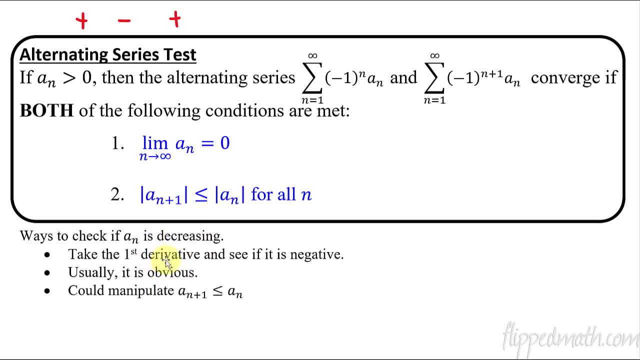 that it's decreasing. How do you know that A of N is decreasing? One way is you take the first derivative, see if the first derivative is negative. I don't like this way because this is the hardest, most cumbersome part of doing it, So I would probably avoid that if I can. 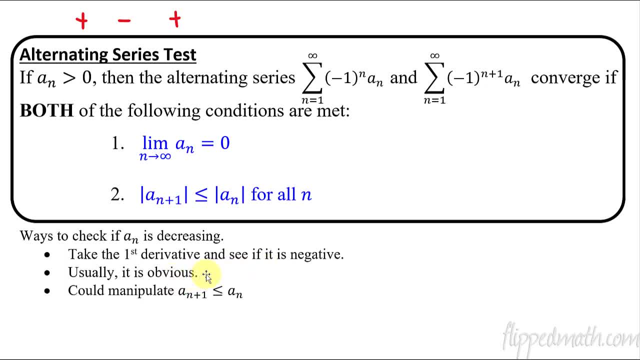 Taking the first derivative to see if it's negative. Usually it's obvious. You'll see what I mean. And that is just that if you look at the, at the value of your A, of M, the expression, you can just plug in numbers and see, yeah, it's going to get smaller. 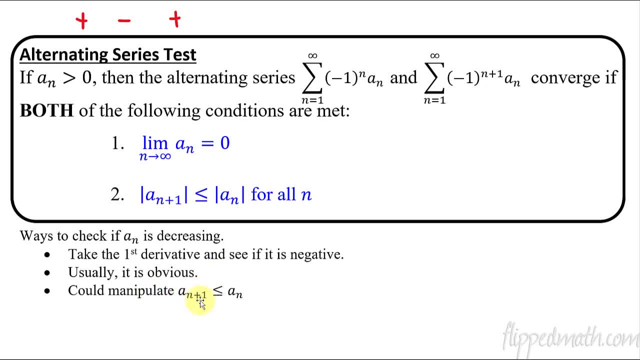 Yeah. And then another way is to manipulate this thing. So if we say that the- the succeeding term is smaller than the previous term, another way of looking at that is one of these two things. you could just say: well, okay, So the bigger term minus the smaller term has to be positive. 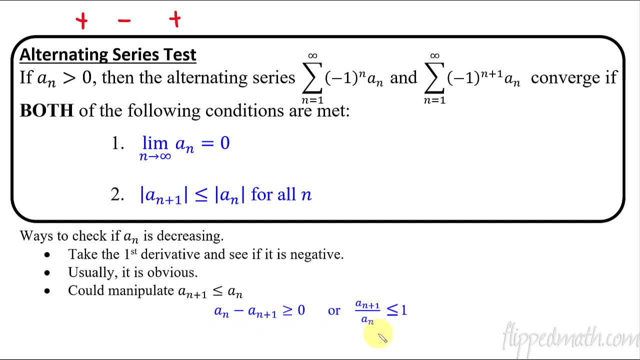 Okay, That's kinda like a no-brainer: The bigger term minus a smaller term is positive, Or this. I like this one: The the uh first term is the denominator of the second term, or the fourth term is the denominator of the fifth term. 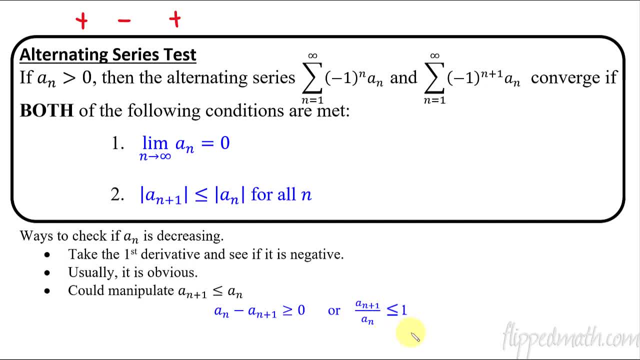 Aquí la 9700 era es un dato original, pero esta es indirecta. Everybody lo que羽ールa para finalizar. If you create a ratio that has to be less than one, That's the only way for that to work out. 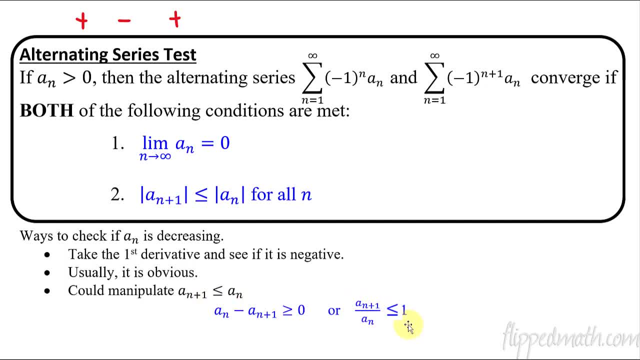 For these two things to be true, this fraction would have to be smaller than one. So I'll do one example of those in these notes here. All right, so get those written down, Let's practice this. So, with our first example, 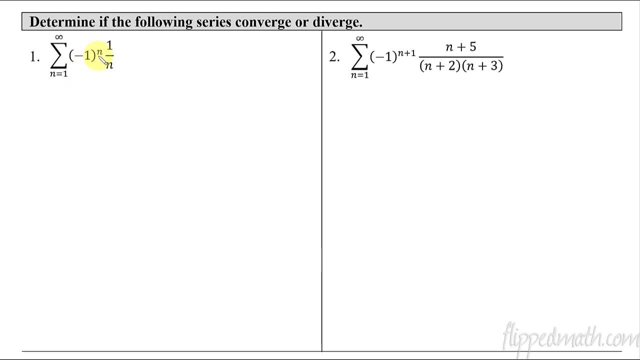 we have here an alternating series. We have negative one raised to the nth power, So it's going to be alternating And so let's check to see our various conditions. Now this actually here. this is kind of cool. This we've looked at before. 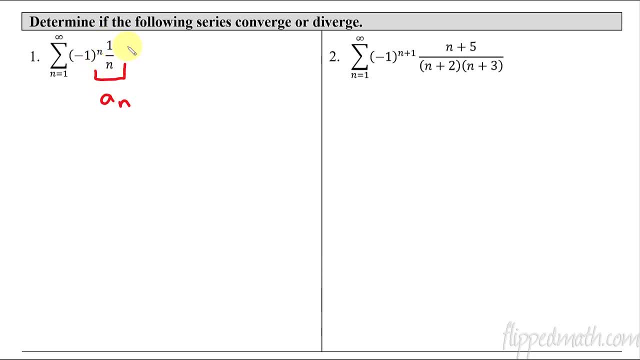 This is harmonic. okay, So this is our a of n and this one actually is our harmonic p-series. We've talked about this. This is called an alternating harmonic, So a harmonic's p-series diverges, That part of it diverges. 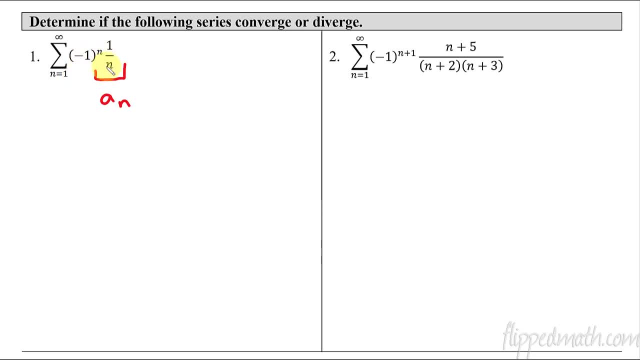 Interestingly, when you create an alternating harmonic, it's going to converge instead of diverge. So here's how we can show that: The limit. do that in blue: The limit as n approaches infinity of one over n. so that is going to equal was. n gets really, really large. 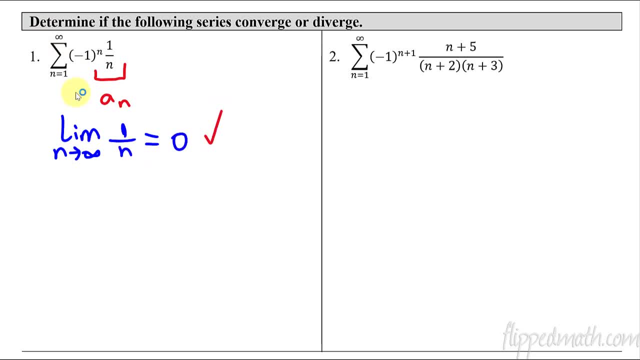 That's just going to equal zero. Okay, so good. Our first condition was met: check, We're good there. So now our second condition: is it decreasing, Is it getting smaller? So one way of checking. that is just if I look at. 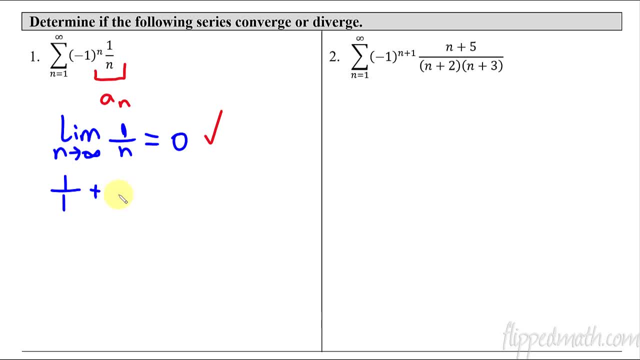 this one's the obvious one. If I just say, if I plug in a one, plus now plug in a two plus, now plug in a three, plus now plug in a four, and so forth, You just keep going and going and going. 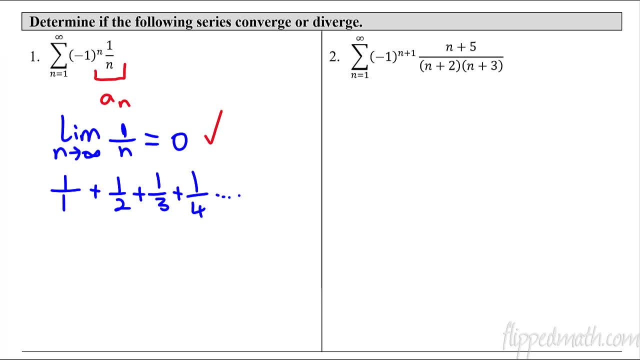 You can see, each one of these numbers is getting smaller, smaller, smaller, smaller. So yeah, this thing is decreasing, Decreasing. So it meets both conditions. It is alternating, So we can therefore say that it converges by the alternating series test. 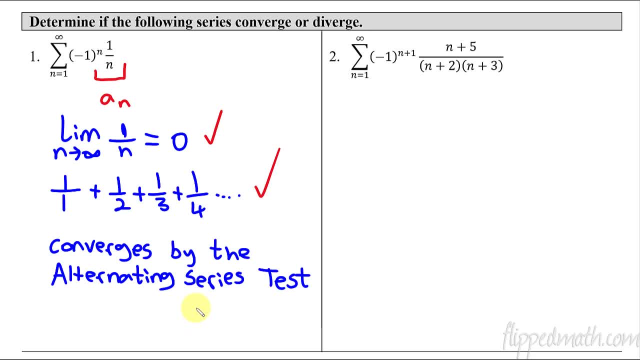 Okay, so we met both conditions. It wasn't alternating And so therefore it converges. All right, so let's try another one here. So this time we have this piece right here. That is our a of n. It is alternating. 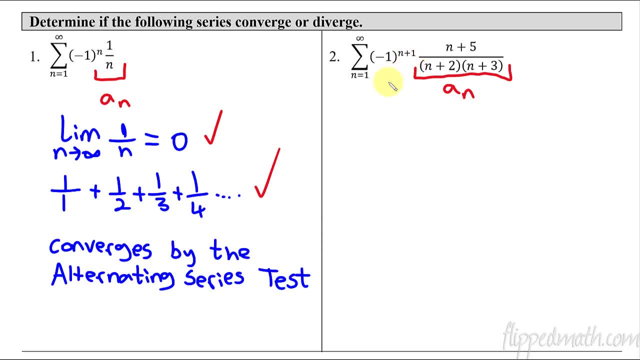 We have this negative one raised to a power Now, just because it says n plus one, that doesn't really change much, except for it's going to start off positive. See, this one started off as a negative number. You plug in a one, it's negative. 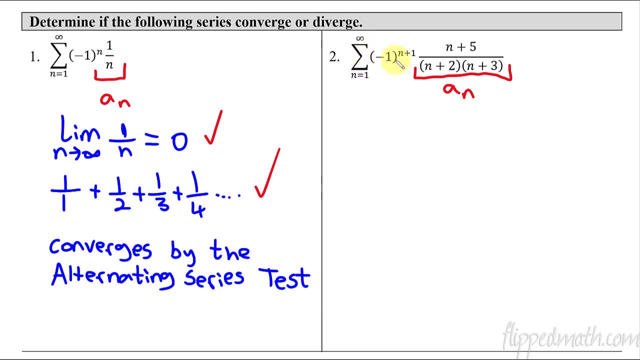 This one. when you plug in the one there, one plus one is two. it's going to make that positive. So that's the difference. When you have an n plus one, it just makes it the first number, whether it's positive or negative. 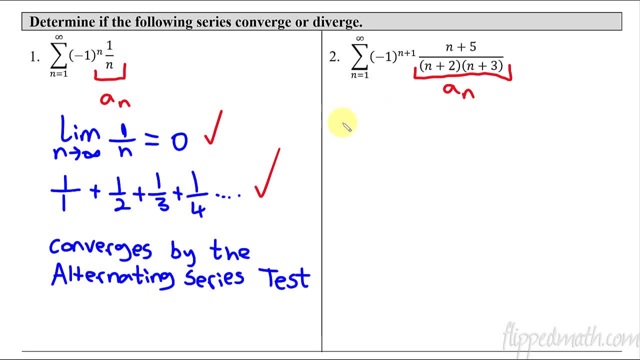 That's how it changes things there. So let's first do the limit, First condition. So I'm just going to write a of n here, a sub n, because I don't want to rewrite that whole thing. So that is going to equal. well, let's see. 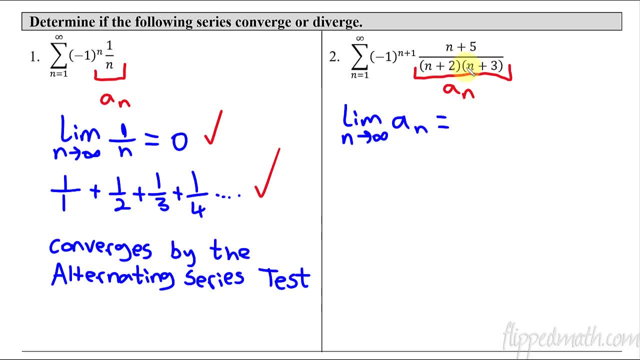 This is the end of the first power. This is going to have an n squared on bottom, So an n squared on bottom with an n on top is going to make this thing approach zero. Okay, so we're good there. First condition met. 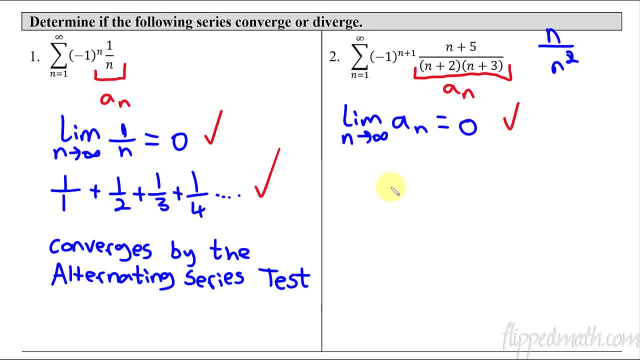 Now what about the second condition? This is where it gets a little tricky. So we could do this thing where I plugged in numbers and I just kept going and going and going and I could show a whole bunch of numbers there, And if I was using a calculator, 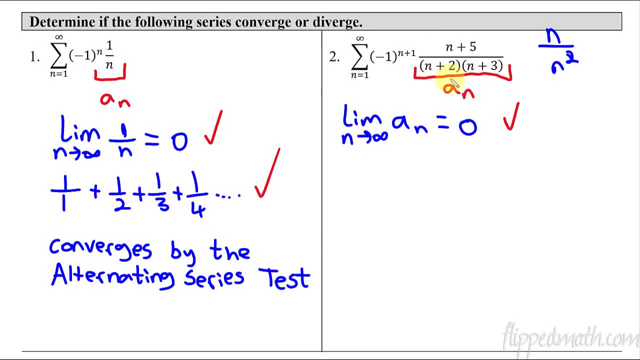 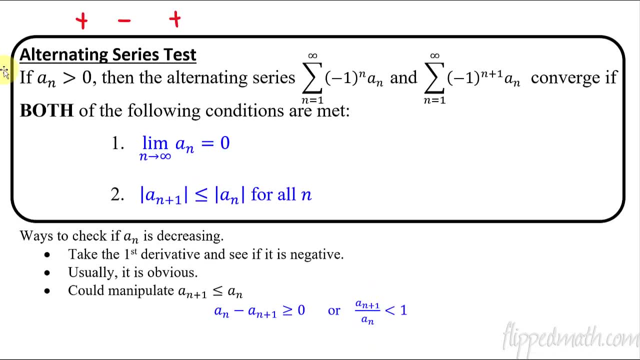 that's kind of a nice thing. I could just plug this into the calculator and check the table I like, using the table function, and check for the table of values. Let me show you this trick here, which was dealing with this one, So I already know what a of n is. 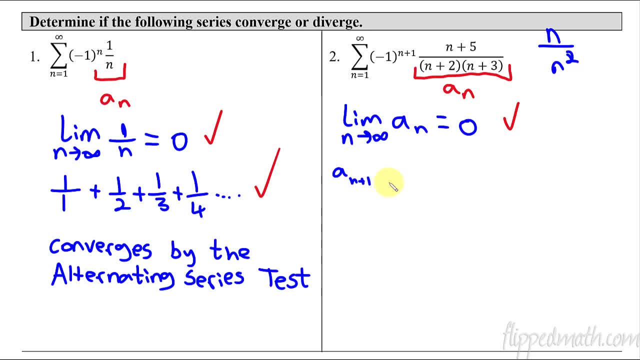 Let's write down what a of n plus one is equal to. So if this n becomes an n plus one, that makes this n plus six. n plus one plus five is n plus six. This one is n plus one plus two, That's just n plus three. 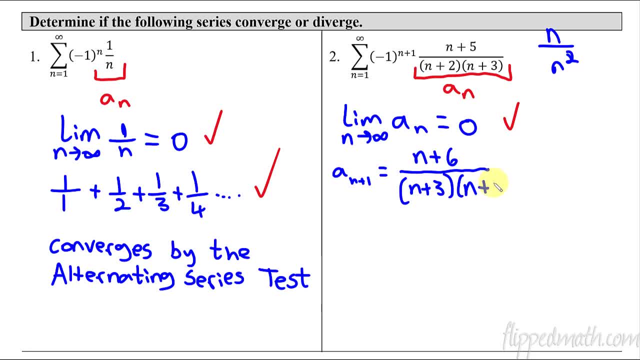 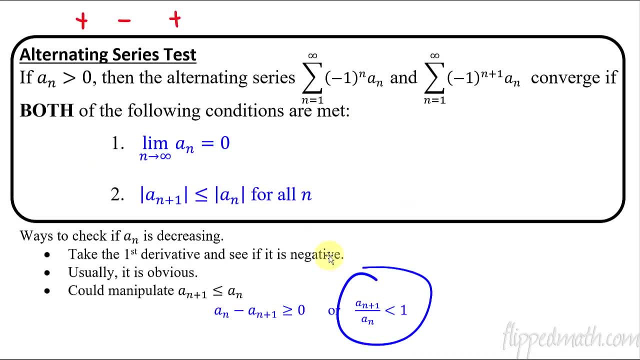 This n plus three now becomes n plus one plus three, So it's now n plus four. So what next? Now we're going to do the ratio. So remember, the ratio was that I'm gonna say a of n plus one divided by a of n. 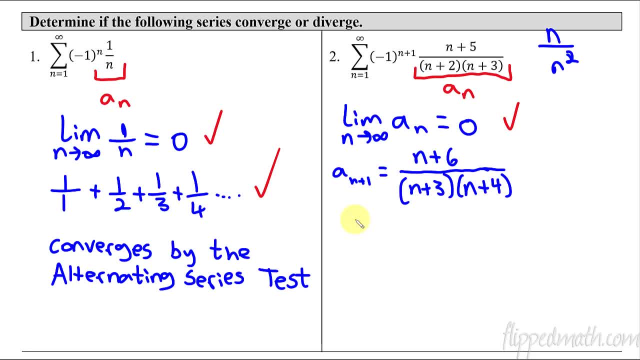 So I'm going to take my a of n plus one, So I'm gonna rewrite this down here real quick: n plus six over n plus three times n plus four. And now, instead of dividing by a of n, I'm gonna multiply its reciprocal. 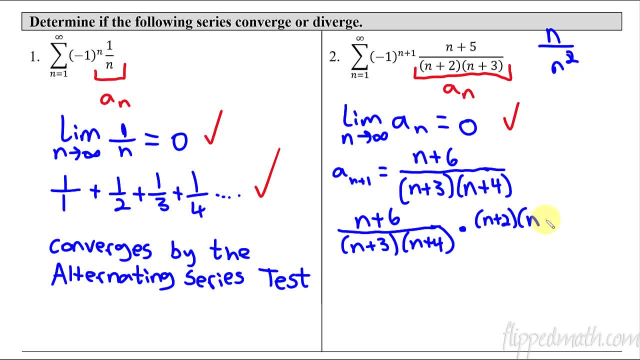 So the reciprocal of this: n plus two, on top times n plus three, And that's all over n plus five. So now let's see, is this thing less than one? Oh, that's really like. how do I know that? 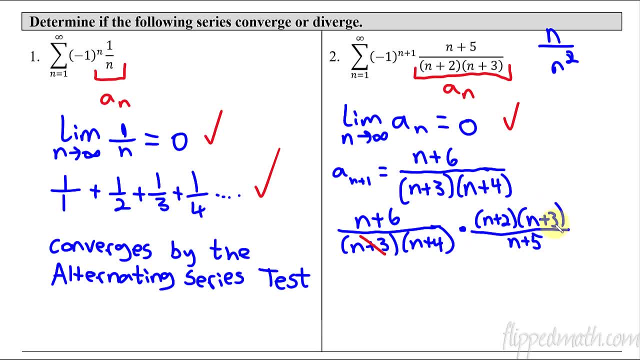 I'll show you. We're going to cancel out the n plus three, cancel out the n plus three, And then I'm going to multiply out long way. So I'm gonna take n plus six times n plus two. multiply that out. 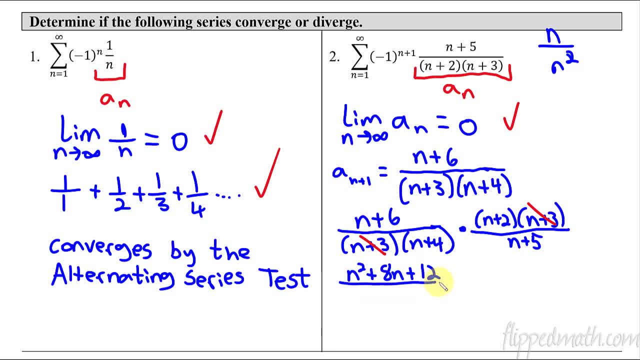 And I get n squared plus eight, n plus 12. And then all over, And now I'm gonna multiply n plus four times n plus five. That gives me this here: n squared plus nine, n plus 20. Now how do you tell if this is actually less than zero? 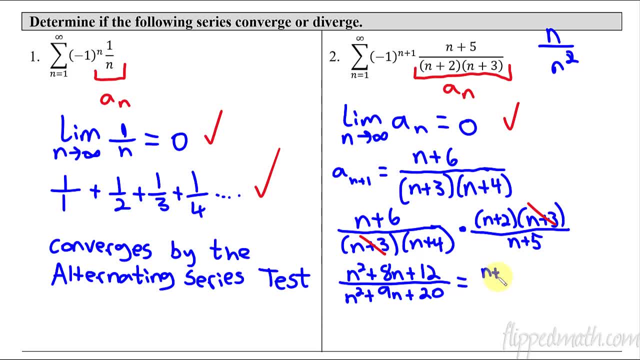 Or, excuse me, less than one. I mean, I'm gonna leave this numerator alone: n squared plus eight, n plus 12.. Now, this is kind of a cool way to manipulate this. If you take this, this is the same thing as n squared plus eight, n plus 12.. 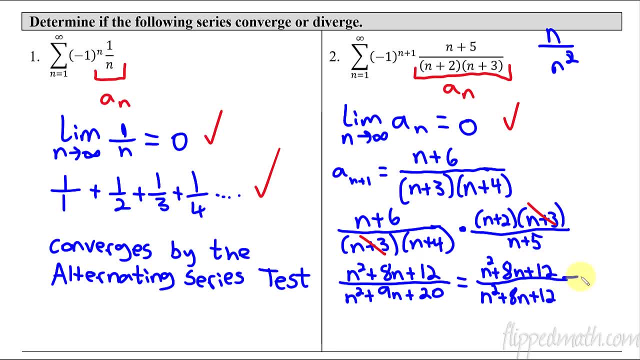 It's going to. I'm gonna write it exactly like the numerator, but then so I have this portion of it plus. so look here I can say one n plus eight. See, that is all equivalent to this denominator. So you can see here. 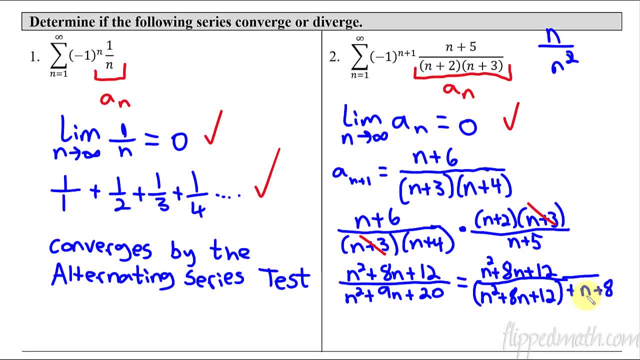 the denominator is the same as the numerator, plus a little extra, plus an n, plus eight. So that's how you can say that, yes, this is less than one, So it meets both conditions And you can say that this converges. 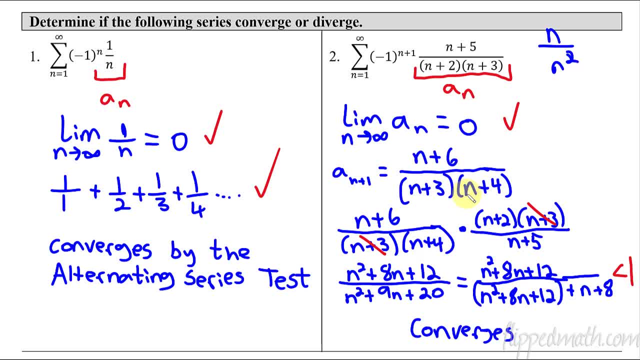 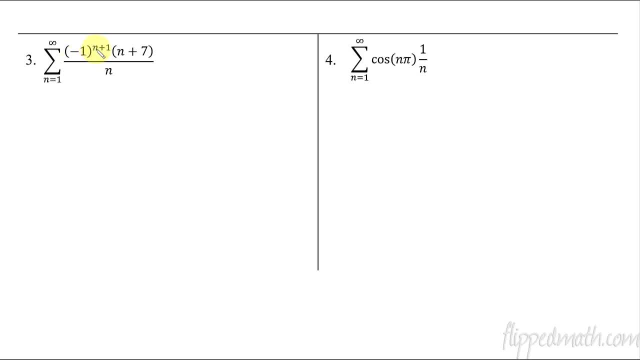 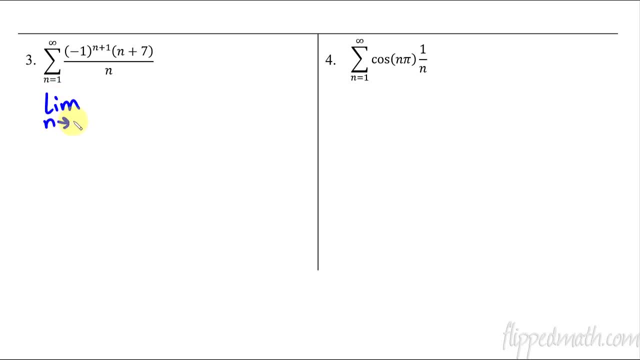 Okay, So now what's my a of n? Okay, So now what's my a of n? That I'm gonna check the limit as n approaches infinity. This one is n plus seven over n. That was sloppy. Let me clean that up. 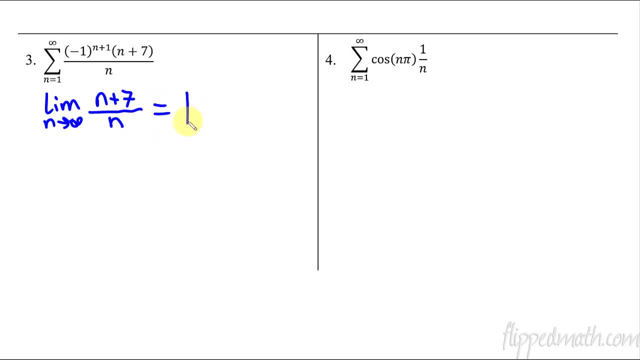 There, that's better. So now, what does this equal? This is equal to one. You have to know your horizontal asymptotes right. We're going off to infinity. This is the first power. This is the first power. The leading coefficients are one. 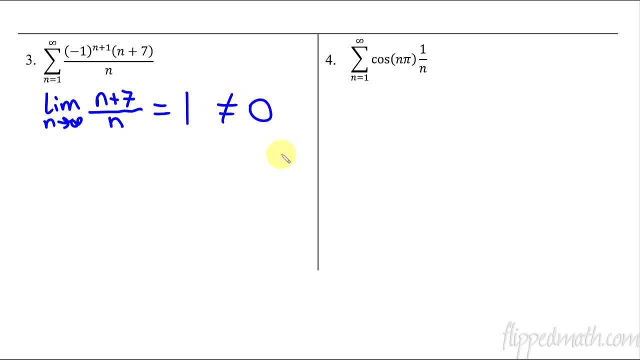 So this equals one That does not equal zero. So therefore we can stop. We don't even need to check the second condition, that it's decreasing or not, Because whether it is or not, it doesn't matter, It does not meet this condition. 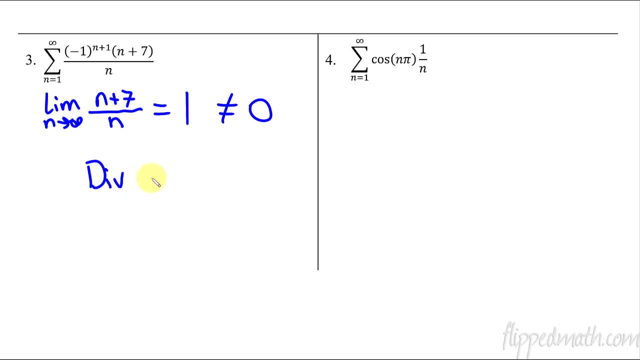 Therefore, this thing is going to diverge and we're done So. it diverges. In fact, if you remember the nth term test, the nth term test, if the limit doesn't equal zero, then we know it diverges If it doesn't equal zero. 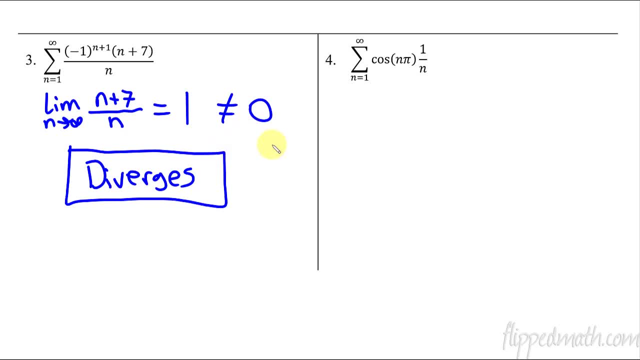 we'd check the second condition. But once the one of the conditions doesn't work, you're done. You don't have to check the other one. Okay, This one here, number four. So when you first look at this one, this is an example of where we don't see. 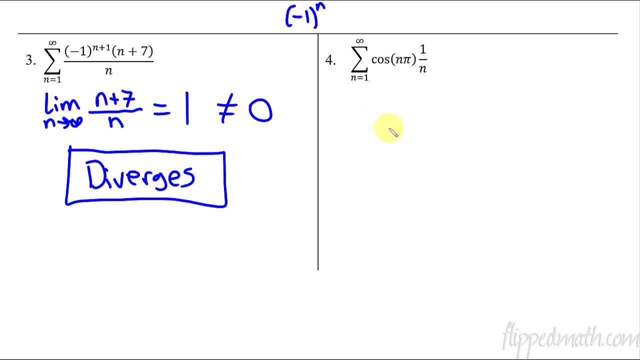 this negative one, raised to the nth term, The nth power. So, when you don't see it, sometimes we think, okay, this must not be alternating then, And so we might approach this differently. but this is an alternating sequence, And the reason is because cosine of one pi. 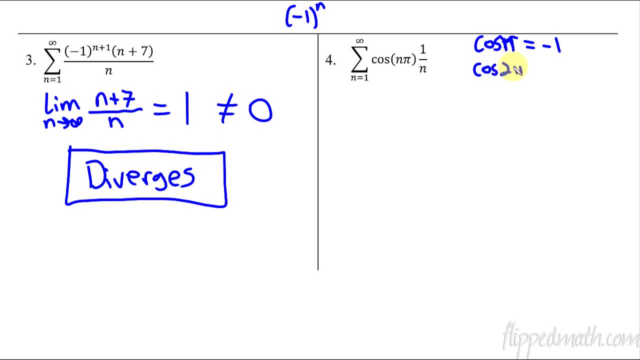 equals negative one. And then, if we plug in a two, cosine of two pi equals positive one, And then cosine of three pi equals negative one again, And it's going to bounce back and forth from negative one to one, negative one to one, over and over again. 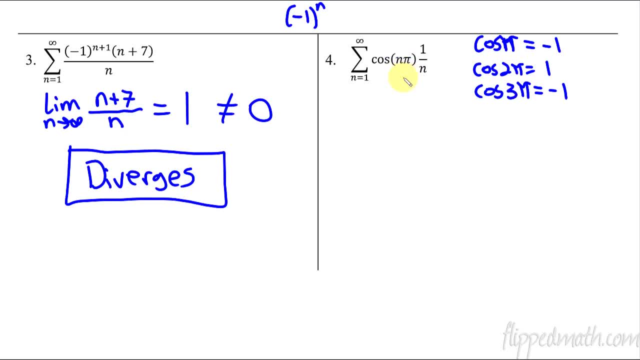 So this right here is the alternating piece, The cosine is the alternating. So since it's alternating, we can go ahead and check our two conditions. So we'll go ahead and do the limit, Because n approaches infinity of the a of n. 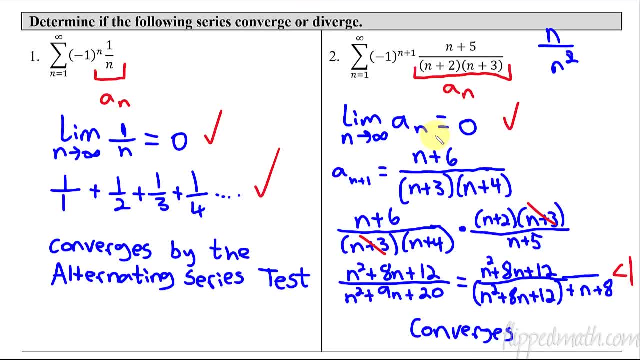 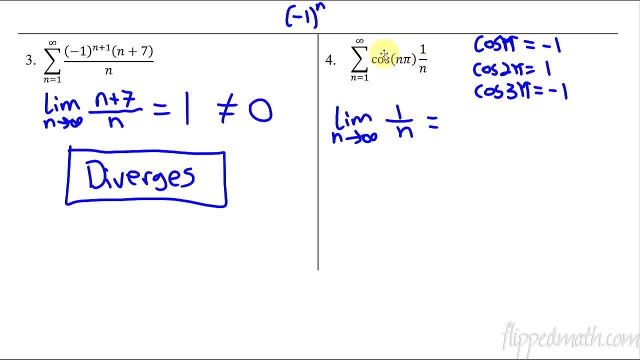 A of n is one over n, which we already did this one. right, That was back on example number one. We did the one of n, So it's actually the same problem as number one, if you recognize it. but now the alternating piece looks a little different. 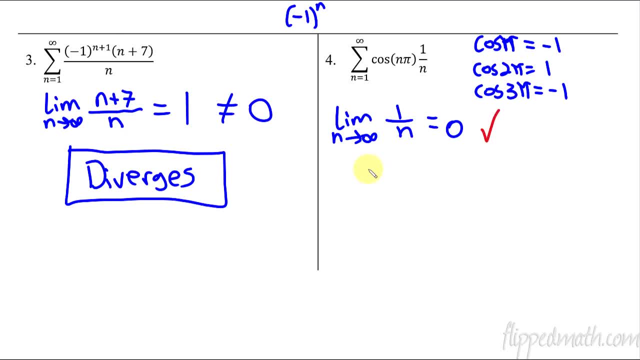 So we said this was zero, So that meets the first condition. And then we know that one over n decreases, it's decreasing, And so we can go ahead and say that this converges by the alternating series test. Okay, so you can see, this isn't too bad. 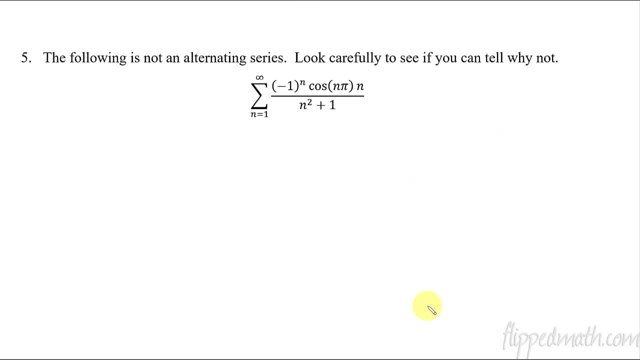 Let's do one more example here, And that is you have one here that actually is not an alternating series. So I would like you to try to look at this and just think about it. So pause the video. Think about why this is not an alternating series.